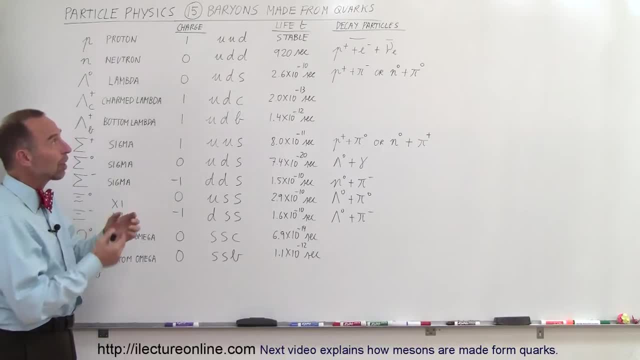 that does not decay very quickly is the neutron. a free neutron will last for about 920 seconds, which is roughly 15 minutes before it decays, and that's a free neutron. a neutron which is contained within the nucleus will typically last a whole lot longer than that which is a 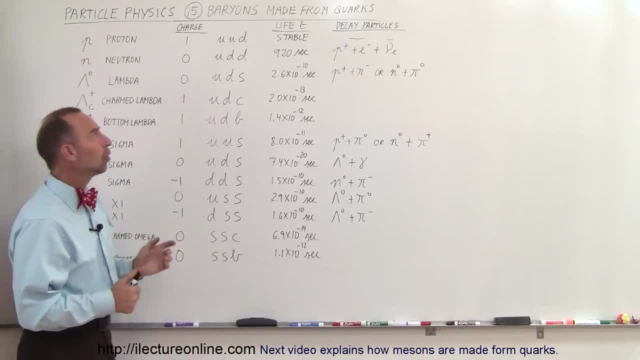 good thing for us, otherwise matter would decay very quickly. So what we can see here is all the various particles that are being formed, and of course, there are several hundred baryons that are created from quarks, and we only have a small subset here. the more famous ones, the 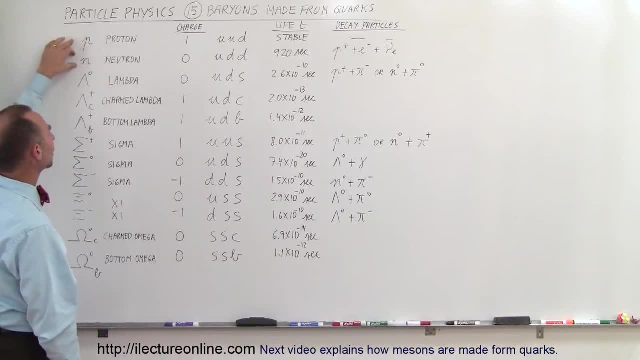 more familiar ones. so we have the proton and the neutron, which make up nuclei of atoms. we have the neutral lambda particle, we have the charmed lambda and the bottom lambda, we have the positive sigma, the neutral sigma and the negative sigma, we have the neutral psi and the negative psi and we have 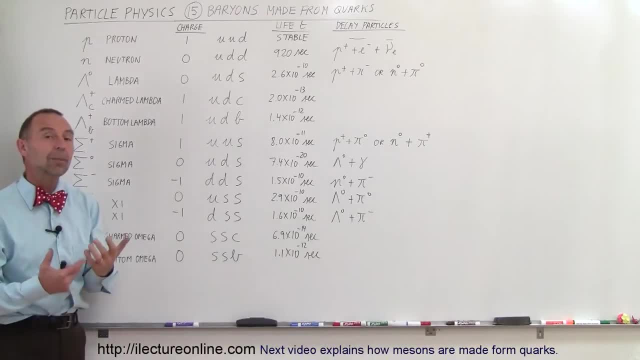 the charmed omega and the bottom omega, and they're just kind of representative of some of the more common particles, Although I would say the charmed and the bottom lambda and the charmed and bottom omega are not as common, but yet you know part of the set that tends to get created when we do a lot of research. 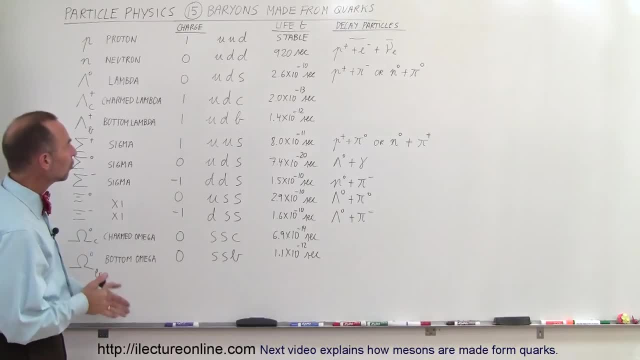 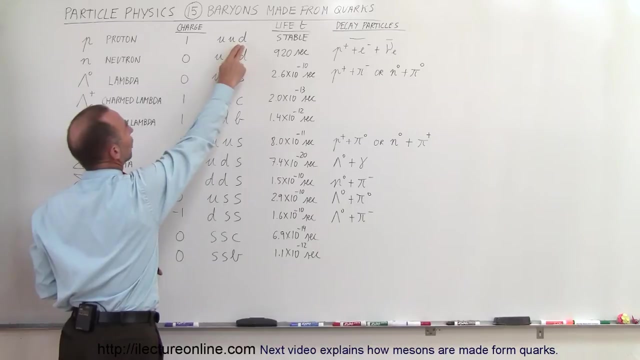 work in our nuclear accelerators. Now notice the charge. either they're neutrally charged, positively charged or negatively charged, depending upon which quarks make up that particular, that particular baryon. Notice that the up quarks have a positive two-thirds charge and a down quark has a negative. 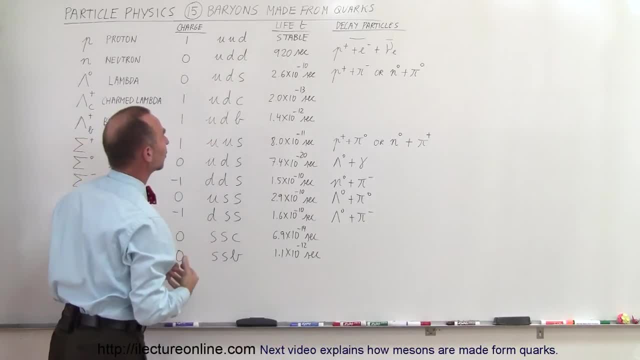 one-third, so positive two-thirds Twice one-third is a positive charge. two negative one-thirds in a positive charge give you a zero charge. You can see that the strange quark has the same charge as a down quark minus one-third. So two minus one-thirds plus up two thirds is neutral. 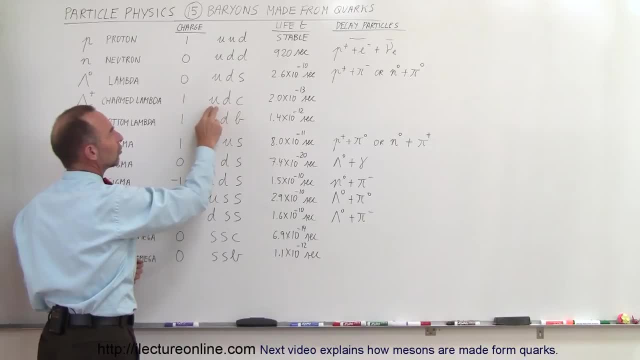 Notice that a charmed quark has the same charge as an up quark, so both of them have a positive two-thirds. So down quark is minus one-third. so together they give us a positive one-chart. and the bottom quark has the same charge as a charmed quark. so again, bottom is plus two-thirds. 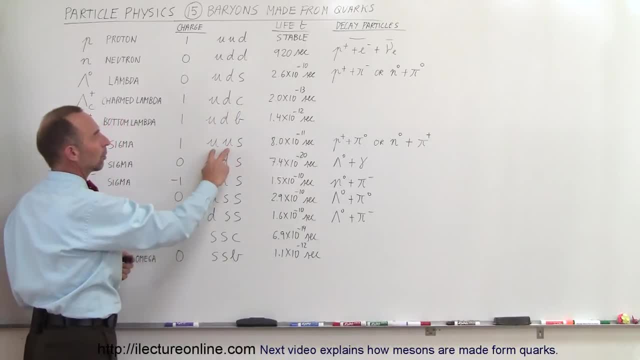 up is plus two-thirds, down is minus one-third. The two up quarks. both are plus two-thirds. strange is minus a third and here plus two-thirds. both of these are minus one-third, so they're neutral. Two downs are minus one-third and a strange is minus one-third. 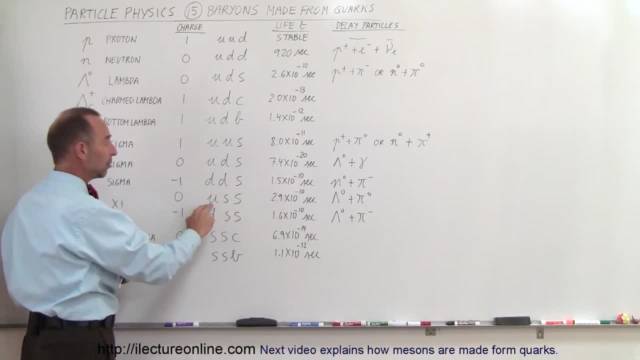 so the three combined form a minus one. The up is a plus two-thirds. each of the strange is minus one-third, so they cancel each other out. The down is minus a third, so are the two strangers. that's minus one, and the charm is up two-thirds. the two strangers are minus a third, so that 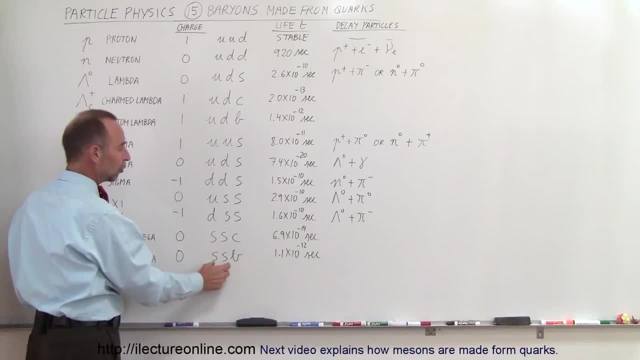 cancels out. The bottom is plus two-thirds, the two strangers minus a third. so they cancel each other out. So that's how you find how the particles that they make up have a charge on them, depending upon the charge of the different quarks. Notice the decay time: A stable particle. 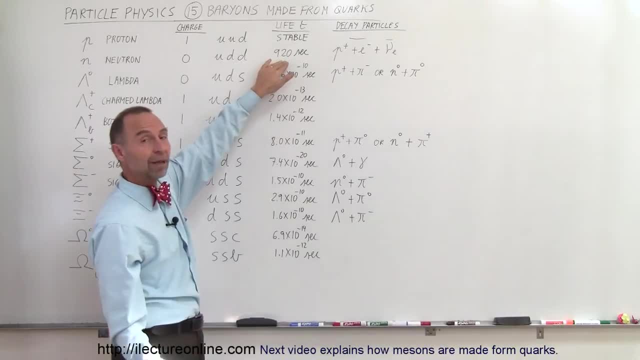 like a proton, will last pretty well forever. Neutrons only last for about 15 minutes in the free format. and then look at the time, The time that these other particles exist: less than one billionth of a second for every one of. 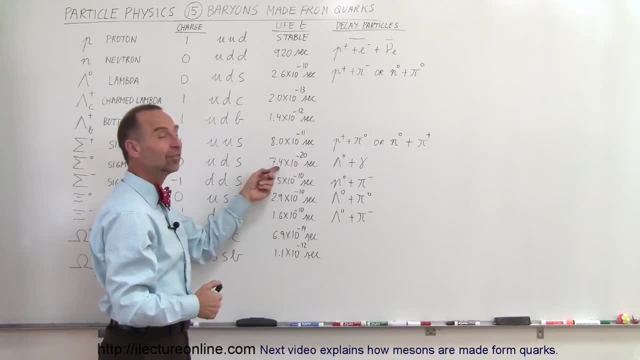 them, In some cases about a trillionth of a second and in some cases even less than that. So these particles are just fleeting particles. Of the several hundred baryons that can be made by quarks, only one is stable. The second one, neutrons, are somewhat stable. Those two particles, 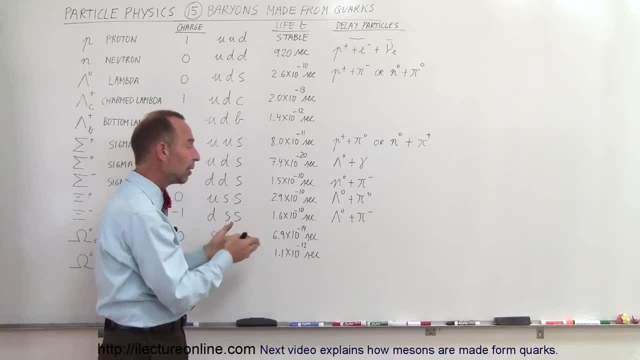 make up pretty well all the visible matter in the universe and all the other particles are just there at very momentary. So you say, well, are they important? They're important in our understanding of the universe. They're important in our understanding of the universe. 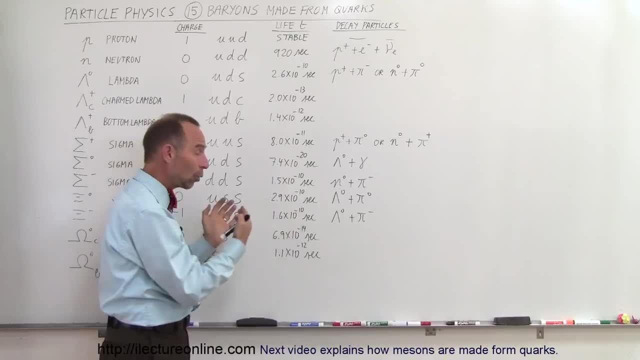 So you say, well, are they important? They're important in our understanding of the universe, They're important in our understanding how matter is made, And you can see that quarks will understand what quarks are and how they behave by looking at the decay time, how long they 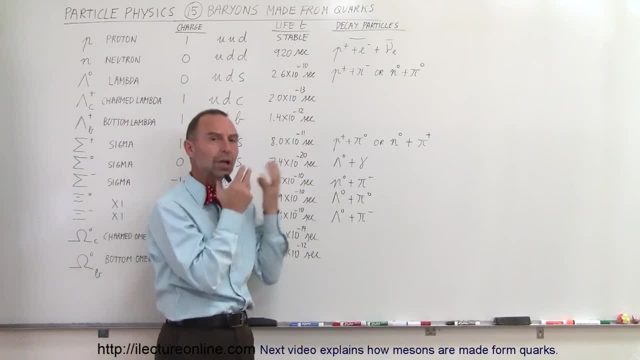 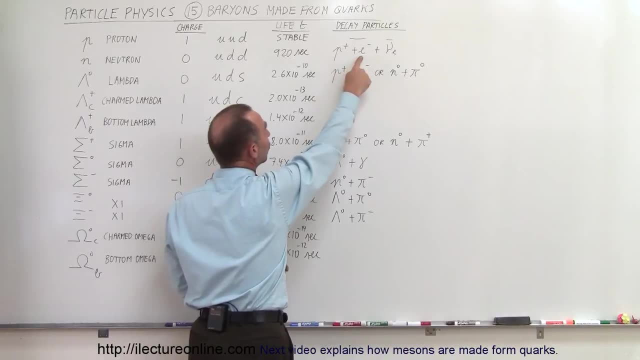 decay and also looking at the decay particles. what particles shoot out from them when they go through their decay process? For example, when a neutron decays, it forms a proton. It shoots out the negative charge from the neutron so that the neutron becomes a positively. 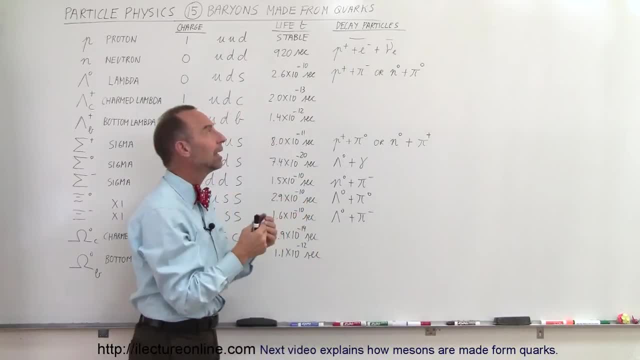 charged proton, and it also shoots out some energy in the form of a neutron, a what we call an anti-neutrino, an anti-electron electron neutrino. If we take a look at a lambda particle, so we can see that it decays into a proton and a negative pion, or in a 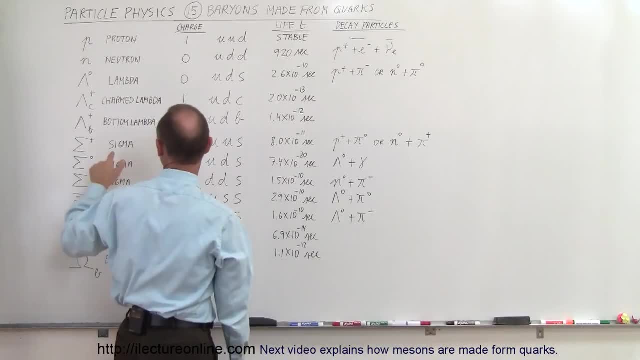 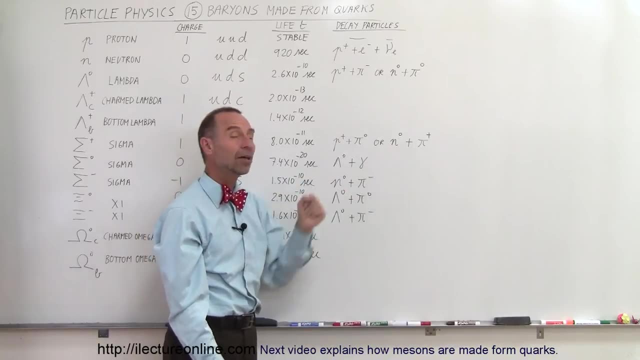 neutron and a neutron pion. If we take a look at a sigma- a positive sigma- it decays into a positive proton and a neutral pion, or a neutron and a positive pion. And if you take a look at a sigma particle, it decays into a lambda particle and a photon. And if you 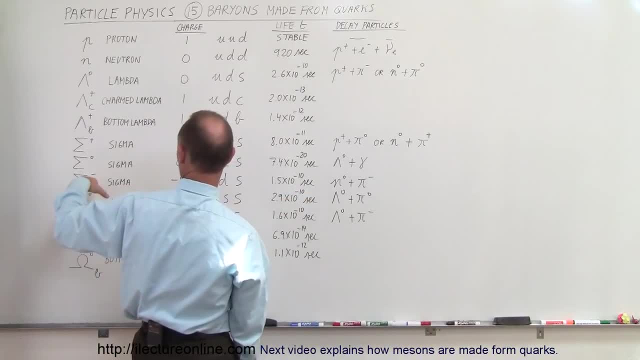 look at a neutral sigma- whoop, I already was there. If you take a look at a negative sigma, it decays into a neutron and into a negative pion and so forth. So you can see that these particles are only around for a very short period of time and they very quickly. 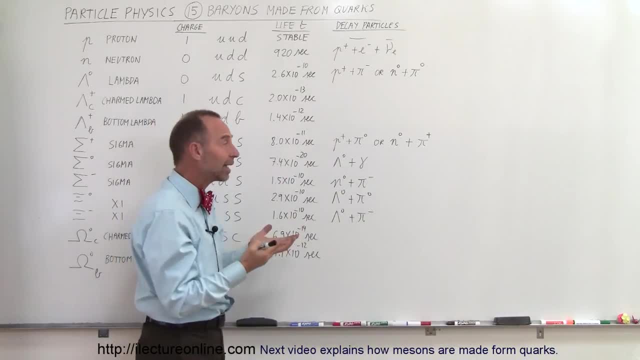 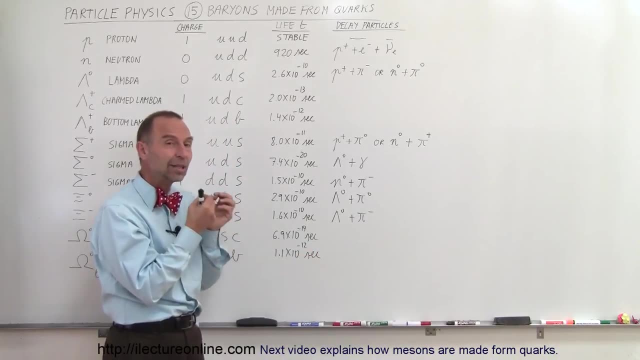 decay into something that's very different. So it looks like all these other baryons, these hundreds of baryons that we've discovered through our studies In the accelerators, are particles that are only there very briefly because of the energy we put into them, and then they very quickly decay to a more stable state and ultimately, 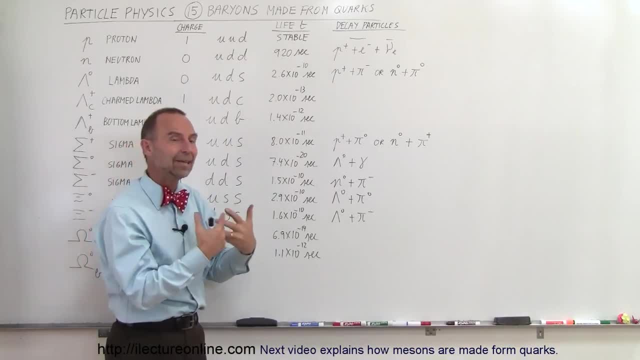 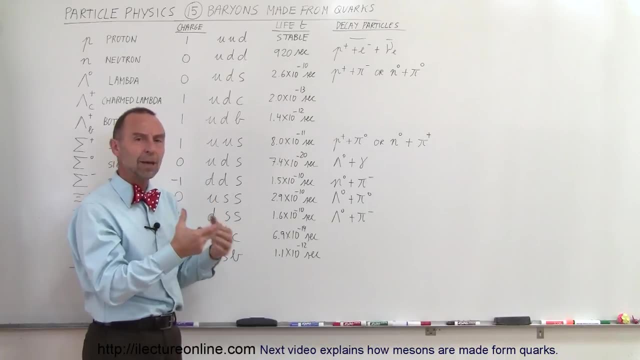 they all decay down to a proton or neutron if the neutron is inside a nucleus. So that gives you a good idea of how quarks work. It seems like quarks were there to make protons and neutrons, and any other particles made from these. quarks are only there for a very 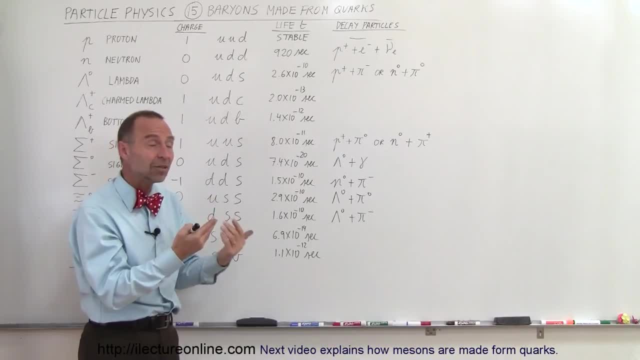 short period of time. In the case of the exchange particles like the mesons, of course they have a real purpose because there's this exchange particle that goes back and forth, so the protons and neutrons and so forth can actually interact with each other. But other than that, there 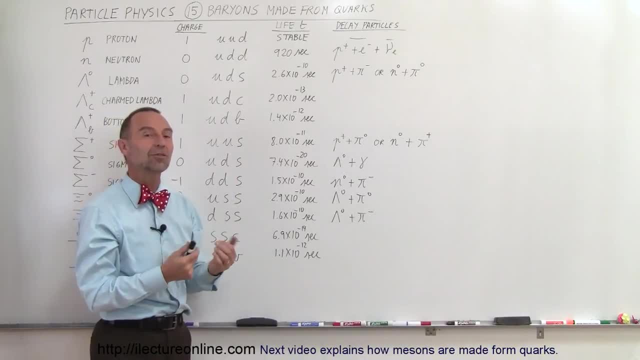 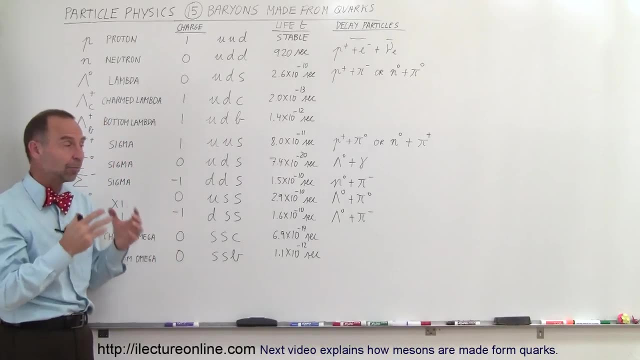 doesn't seem to be a lot of purpose for some of these hundreds of baryons that are only there for a very short fraction of time. So hopefully again, that gives you an idea that quarks are there to make baryons, particles made up of three quarks and that usually